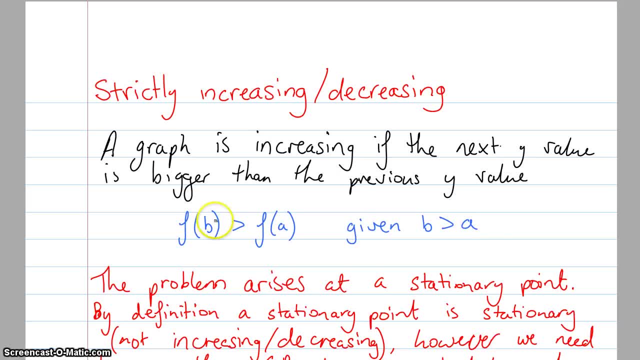 If b is bigger than a, then what we're asking is: is the y value when x is b bigger than the y value when x is a? If that's the case, then we can assume that this graph is increasing. If I go back to my drawing again, I'll draw it up again If this is b and this is a. so 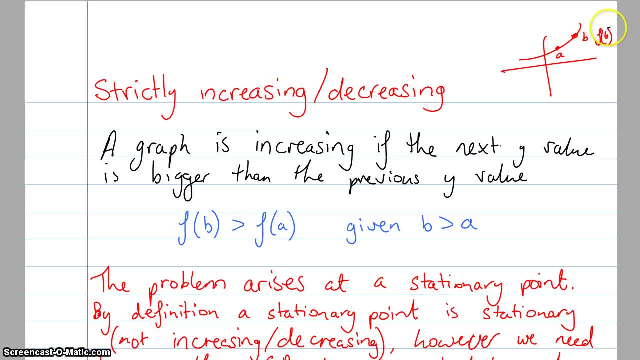 b and a and then we say f of b is bigger than f of a. So it's getting a bit squished, but hopefully you can see. And f of b is bigger than f of a. that means that it's an increasing function, okay, between. 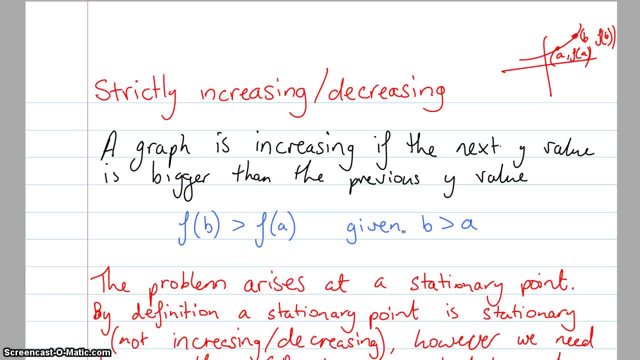 you know a and b, I guess, And likewise you know if f of b is less than f of a. when b is bigger than a, then that means it would be a decreasing function. okay, The problem arises at a stationary point, and this is why this whole thing has kind. 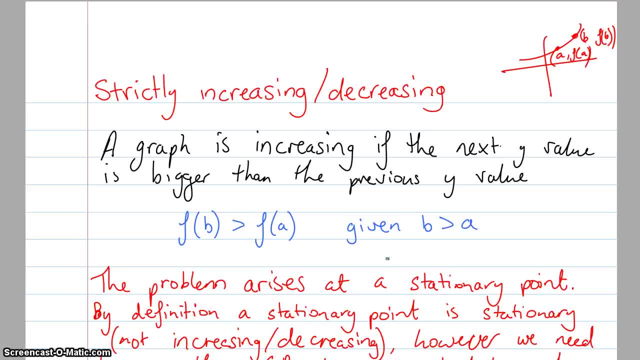 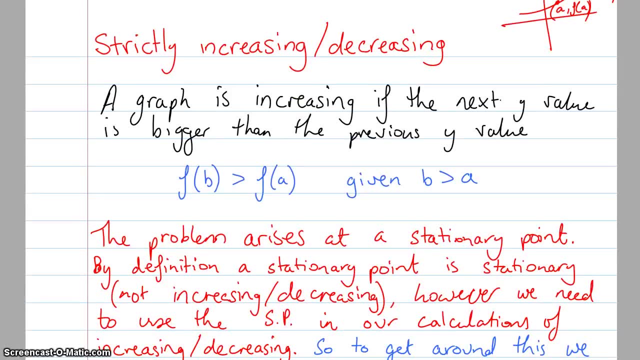 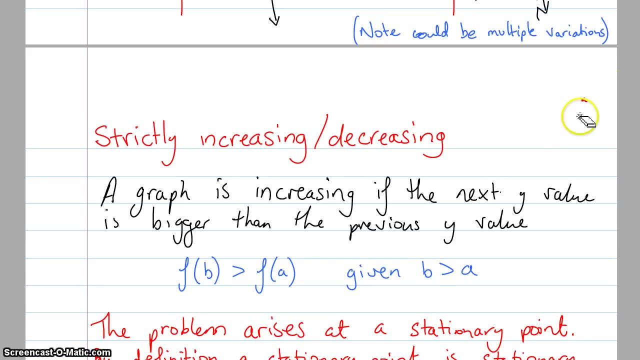 of come in, I guess, because by definition, at a stationary point it's stationary, It's not increasing or decreasing Um. So we need to use the stationary point in our calculations of increasing and decreasing. okay, So maybe if I draw- and I'll get rid of this- and if I draw um one with a stationary point, 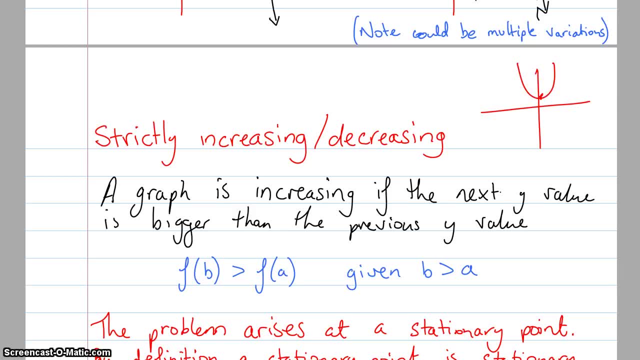 like that. I know that it's stationary. at that point there, when x is zero, It's stationary, It's not moving up or down. But what I want to do is I want to use this point to work out whether the right-hand side 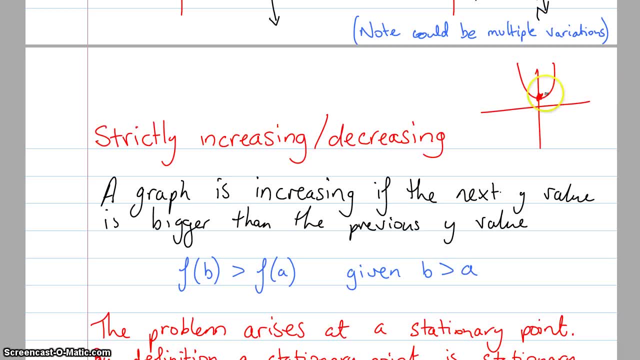 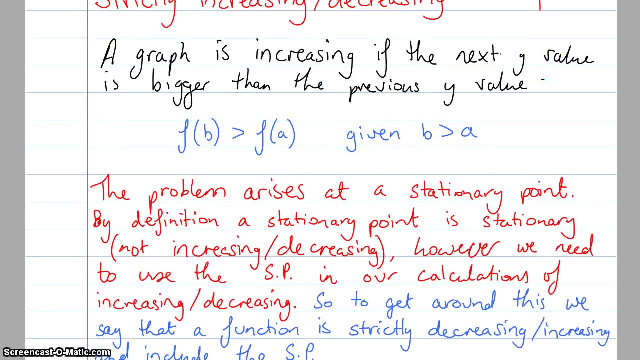 is an increasing function or a decreasing function, And so this is where the confusion comes in, because I actually want to use this, So I'm going to use that point So to get around this idea- and I'll show you an example later on- to get around this. 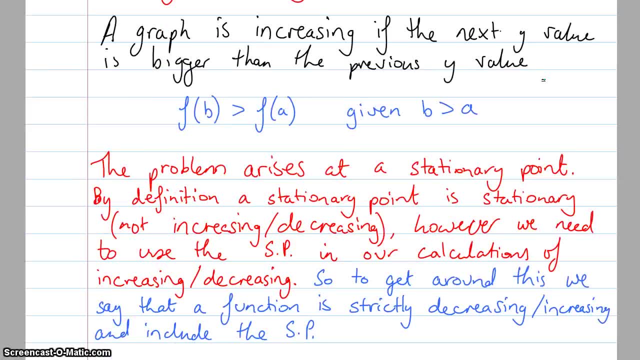 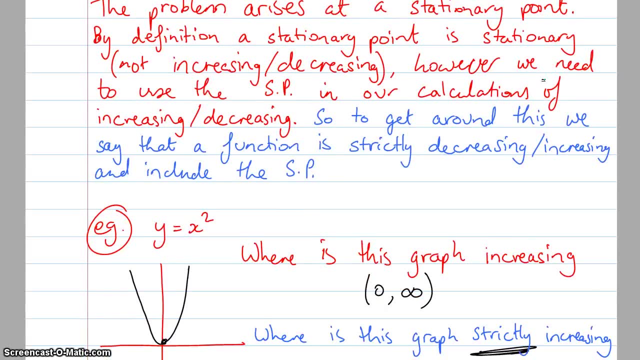 we can say that the function is strictly increasing or decreasing, and that will include the stationary point. okay, So let me hopefully it'll all come together when you actually see this here. So I've got y equals x squared as my graph and I'm asking the question: where is this? 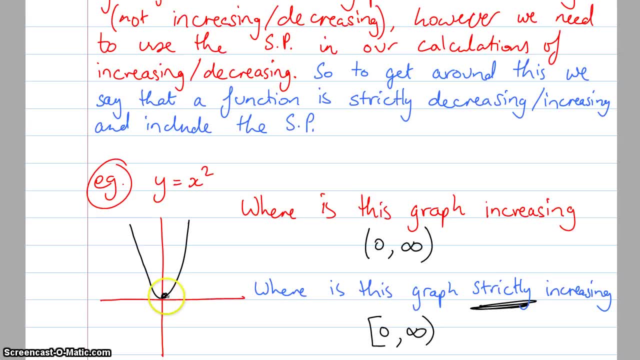 graph increasing. Okay, Well, this graph is increasing, as in the y, the next y values are bigger than the previous y values From zero, So all the way up to infinity, but not obviously not including infinity and not including.